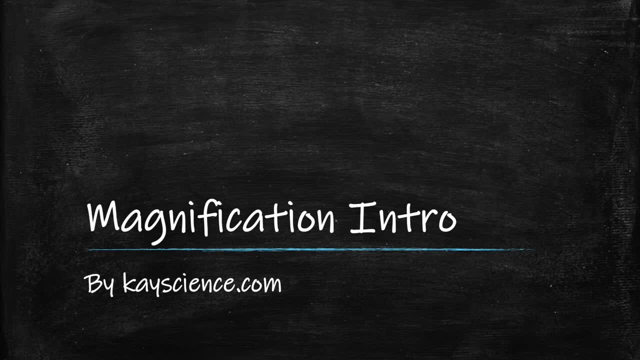 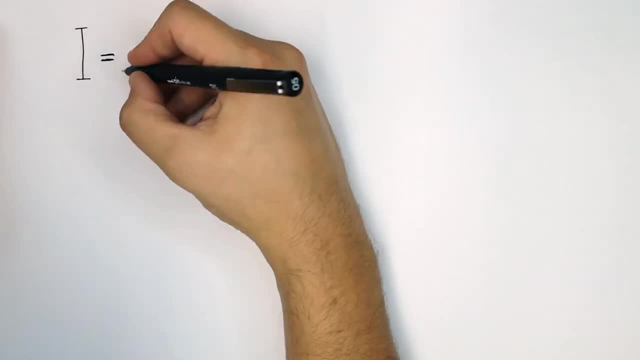 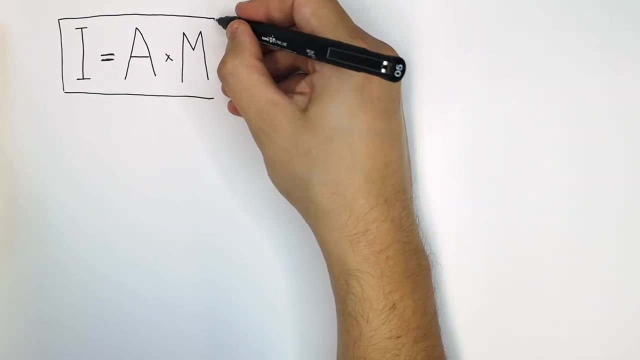 An Introduction to Calculating Magnification by ksciencecom. In calculating magnification you always write I am. I equals a times m. I am equals between the i and the a and the times between the a and the m. So the i is the image size. 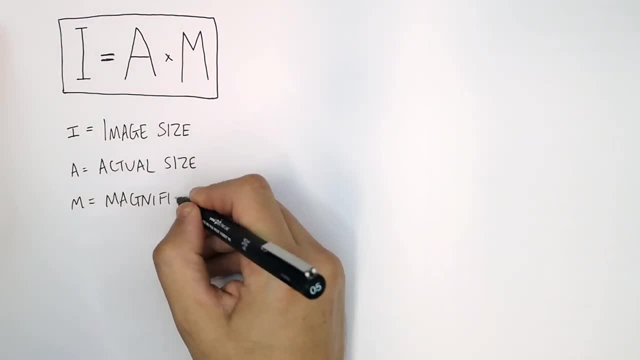 the a is the actual size, the m is the magnification. So then, what you can do is this: you can make the triangle by putting the i over the a times m, which gives you the triangle. So now you can rearrange for any subject. 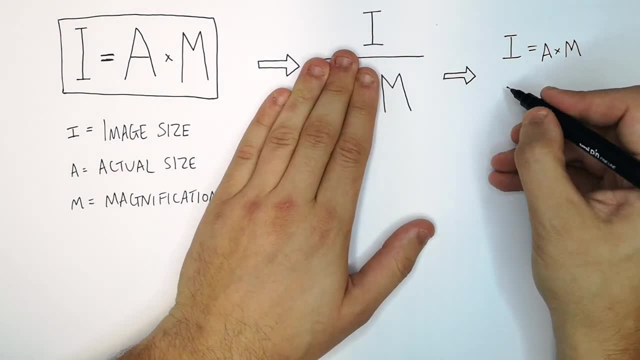 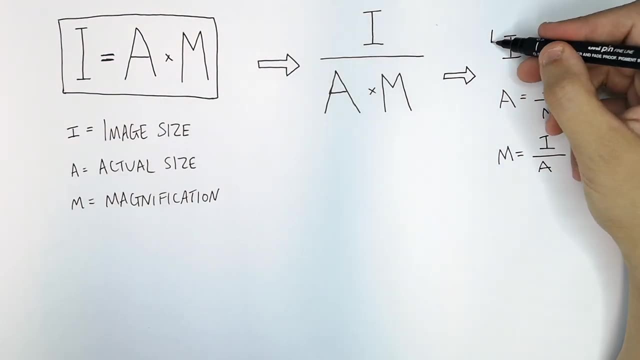 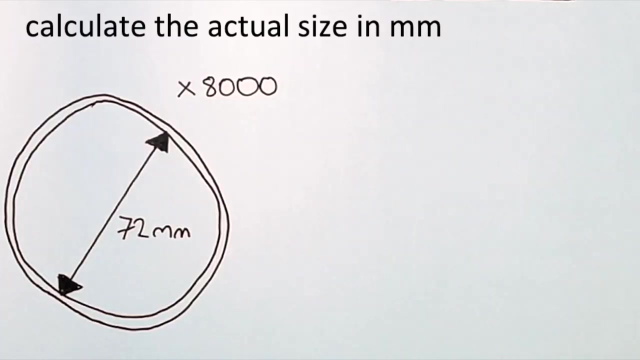 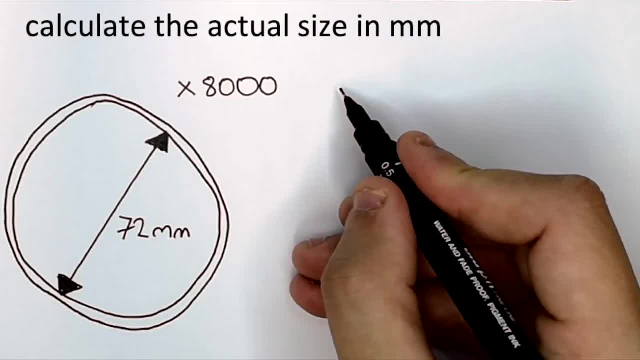 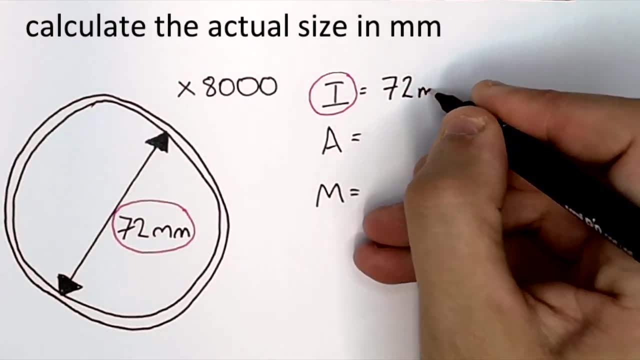 Pause the video here to try and calculate the a times m. So now you can rearrange the formula to make any letter the subject. The first thing you do is write: I am going down, Then you can fill in what you've got. You've got the I, which is 72 millimeters. You've got the M- magnification, which is. 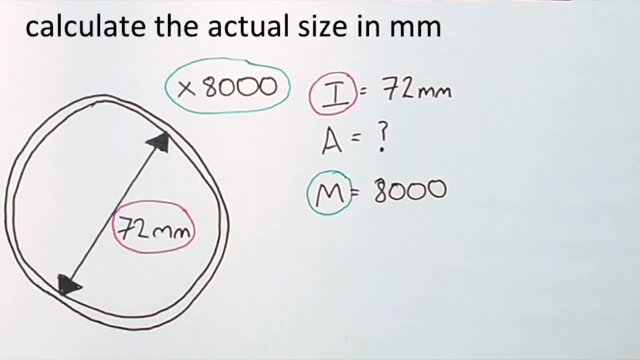 8,000.. So what is A? A equals I divided by M. So then, what you do is simply write 72 divided by 8,000.. So you're dividing I by M, which will give you A, In this case A. 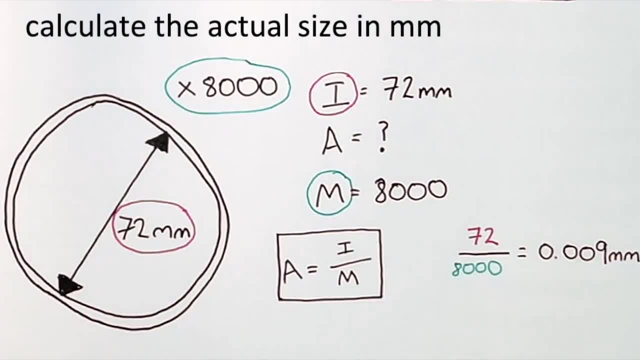 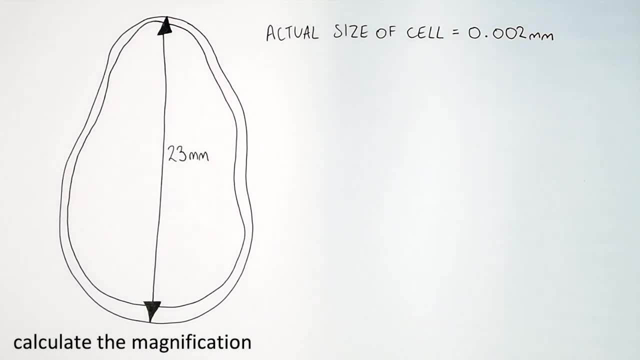 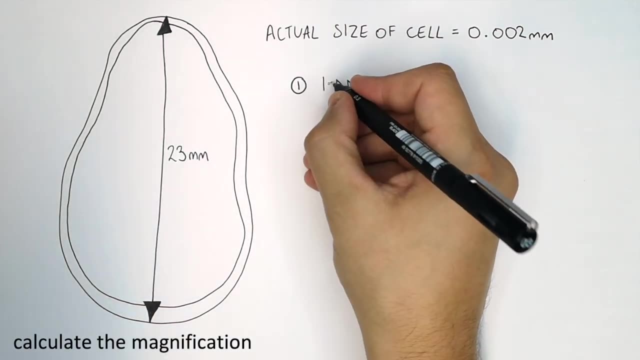 equals 0.009 millimeters. If you think you can calculate the magnification of this cell, pause the video. If not, I'm going to show you how to do it. First thing you must always do is write: I am. Then you can put the equals between the I and the A and the times between: